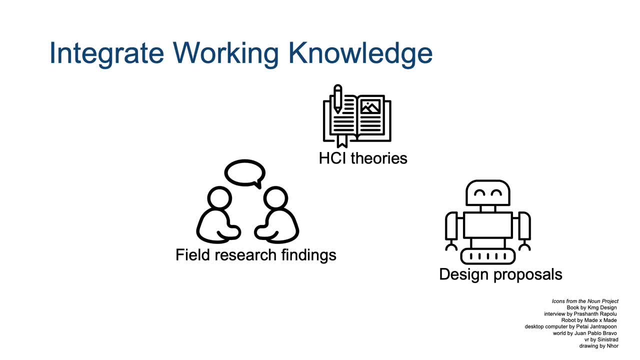 In our HCI classes we often notice a discontinuity between field studies and design properties. Students often make leaps to design that seem to miss out on really interesting design problems and opportunities that they identify from their field research. Theoretical concepts are also often overlooked because they cannot be easily applied to the 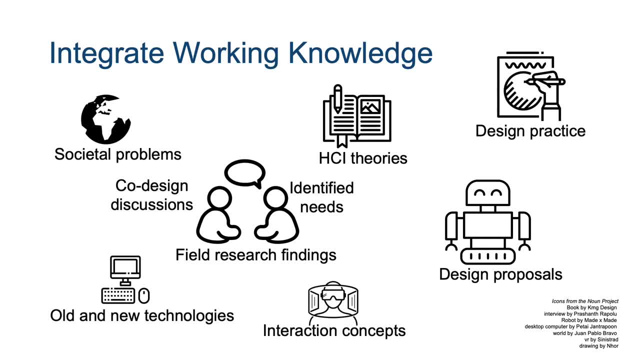 problem at hand. In HCI, designs are also often inspired by larger societal problems, as well as by established design practices, older and new technologies and emerging interaction concepts. So working field theory really integrates all of these concepts. It also creates these insights to highlight opportunities for the design of interactive 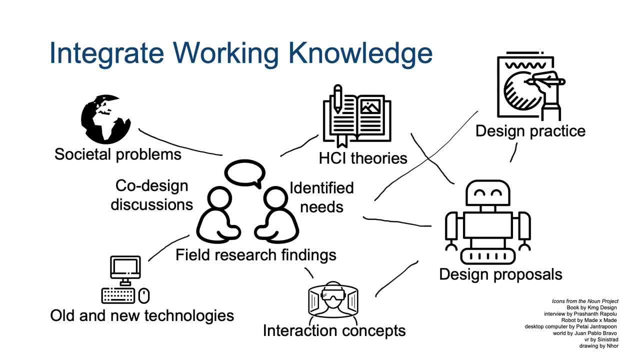 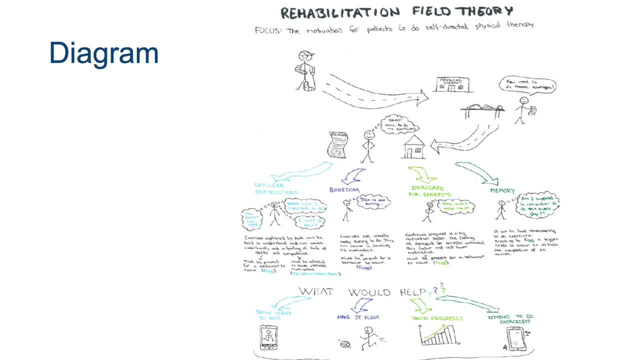 technology. I want to emphasize that field theories are working theories, Humble theories for a particular context, based on a small set of participants, without making any claims for substantive knowledge. In this paper, drawing a field theory diagram is really important to synthesize different. 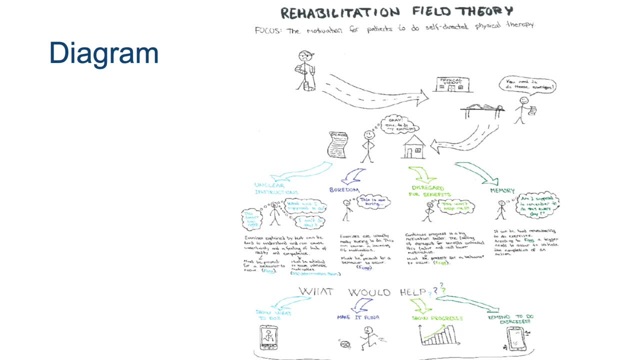 insights from the field and from HCI theories. This diagram was created by students based on field research for physiotherapy patients. It is a nice illustration of field theory. It illustrates key components of a field theory diagram. It fills roughly one A4 page to give an overview of important problems and opportunities. 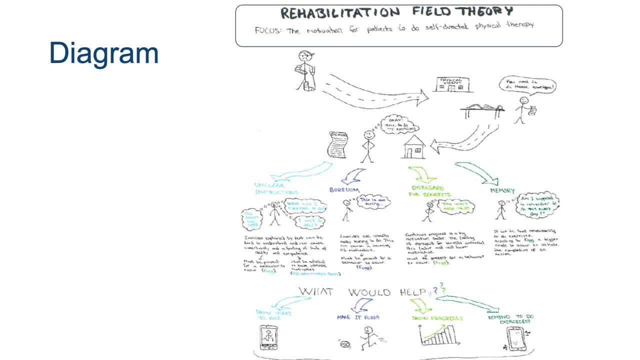 It includes a title and a succinct definition to frame the field theory. Here, the focus is on supporting patients to do self-directed therapy at home, And this is followed by a visual representation of empirical insights. For example, one of the challenges was that exercise instructions were not clear when 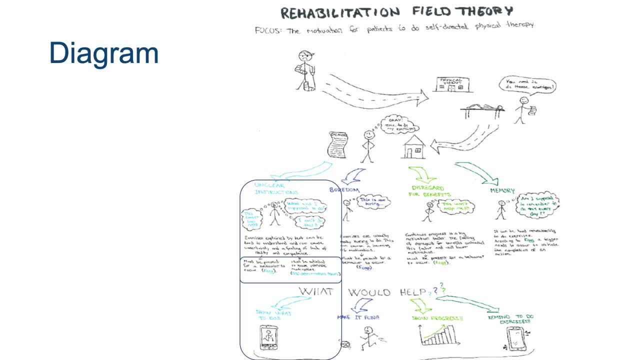 patients tried them at home, And this is why field theory is so important. Participants said that they didn't know if it feels right and if they pushed themselves hard enough, So the diagram also integrates competence and motivation as concepts from self-determination theory. 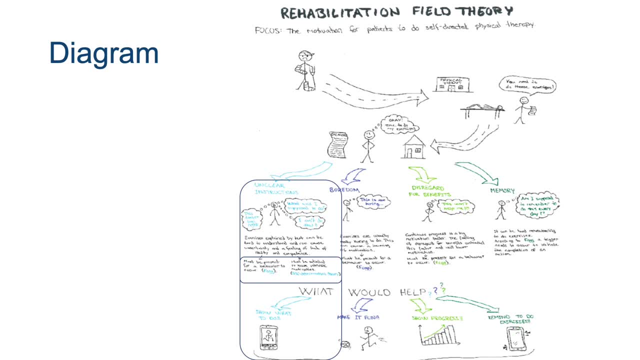 And on the bottom it highlights paths for design, for example, to show more clearly what to do when doing exercises at home. So this example is presented as a patient journey. However, there is no fixed diagram structure. Field theories are really flexible in the way that they can be visualized. 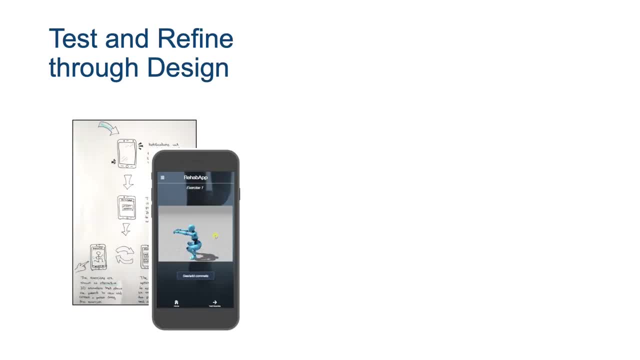 For example, on my own example, according to my students, I have a man sitting in a chair. he has a very sharp eye, The design is very simple and the perspective is very practical, And the students are able to analyze the project in turn. 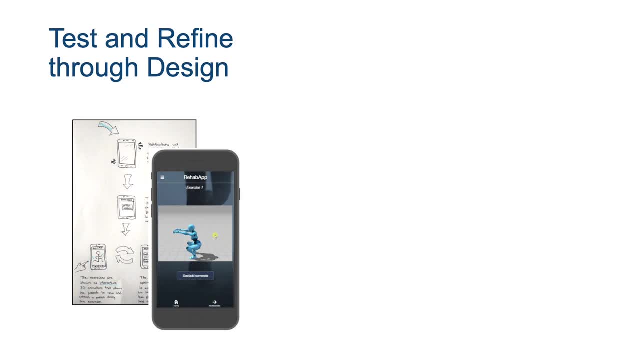 Based on their theory, students develop a prototype design and trial it with two participants. By seeing how the prototype is used in real life, students can test and refine the field theory that framed their design. This also stops students from presenting the design idea as a marketing pitch. 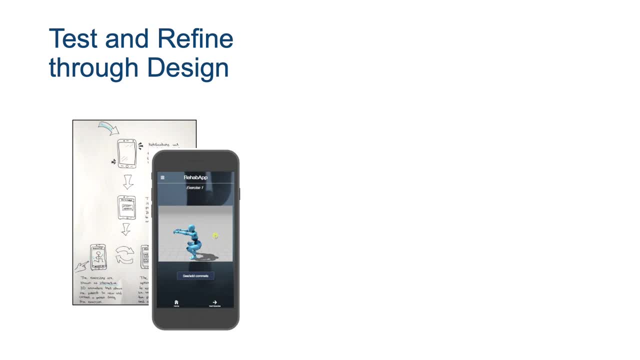 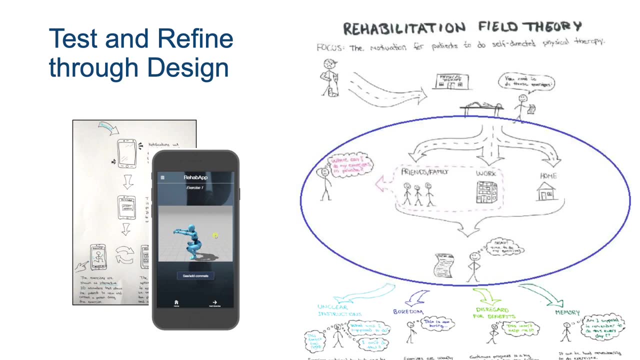 Here's an example. On the left we can see sketches and a prototype mock-up. based on a rehabilitation field theory, this VR prototype was to provide a full body view to help patients remember how to perform exercises. On the right, we see how trialing this prototype shed light. 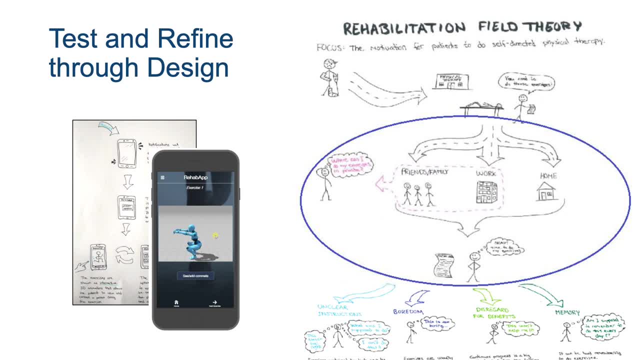 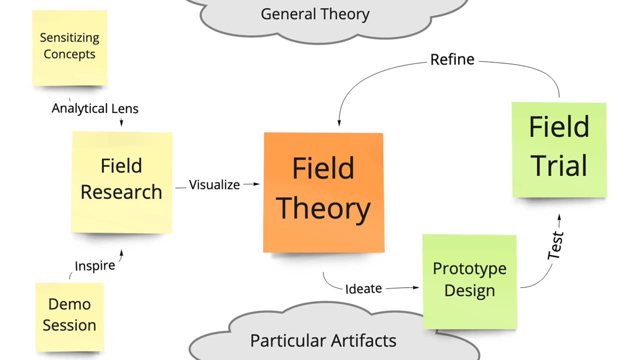 on the different exercise contexts. as highlighted in a blue circle, Participants commented that they would use it at home, potentially also at work, but only if they had a private space. This diagram shows how we approach field theories in the classroom over the course of a semester. From left to right, you see the 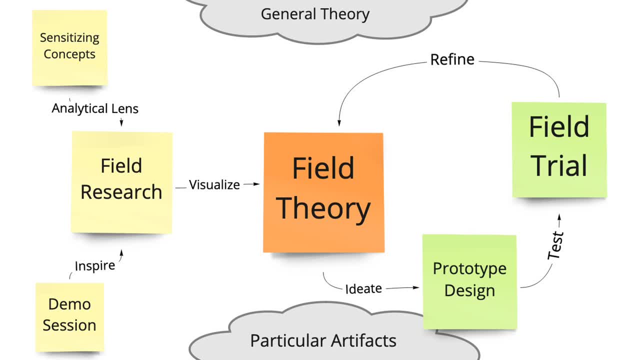 different design research activities. We start with sensitizing concepts and technology demo sessions to really inspire our students. This is followed by research and the field and the visualization of an initial field theory. The paper describes this in more detail. It presents the perspectives of students. 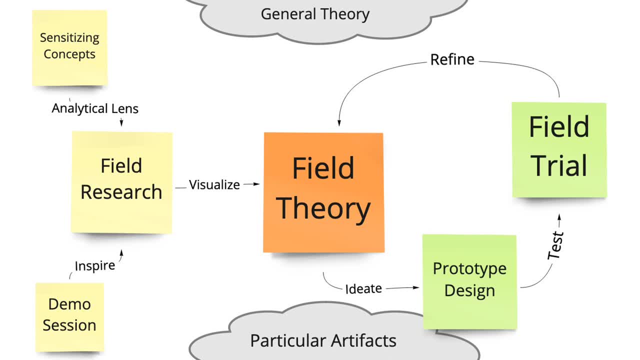 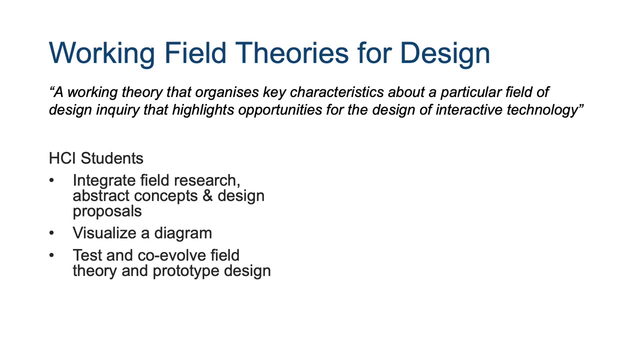 whom we interviewed. It includes our own reflections on teaching field theories over the last five years and, of course, the examples of field theories and prototype designs. Achieving mastery across fieldwork, theory and technology design is certainly an art that requires practice and experience. Creating a field theory helps students to gain such 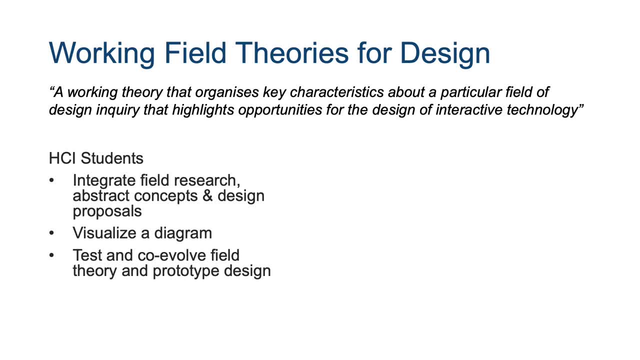 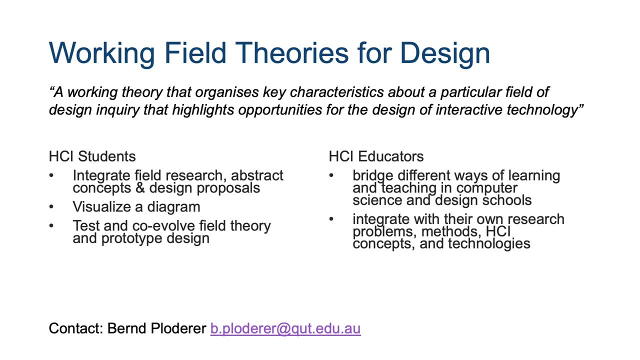 experience. Field theories help students to integrate their field research, abstract concepts and design proposals. They help them to create diagrams that synthesize key insights and help them to test and refine the field theory for a prototype design. In the paper we also discuss opportunities for HCI educators. If you're teaching HCI, 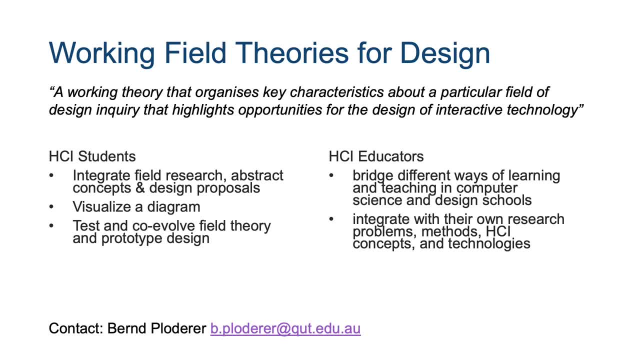 we hope that field theories help you to bridge different ways of learning and teaching between CS, computer science and design schools. In particular, we think field theories help to incorporate creative design principles of ideation, visual thinking and divergent thinking with the traditional iterative design. 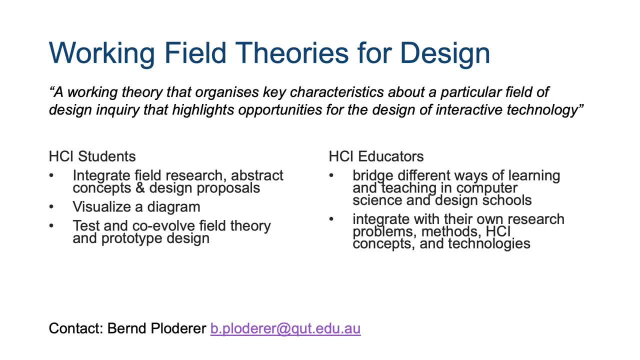 process in computer science. It's also an approach that we tried with different research problems, methods and theories over the years and we are confident that, if you're interested, that you can incorporate it with your own methods, theories and technologies. Thank you.